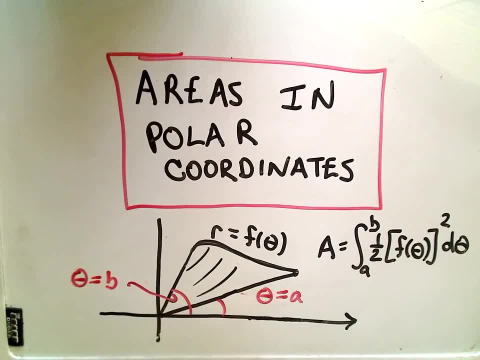 Okay, this video is going to be about finding areas and polar coordinates And to me, I think the tricky thing about these problems- for most people- myself included, because I don't do them that often- is coming up with a decent graph and finding the limits of integration. 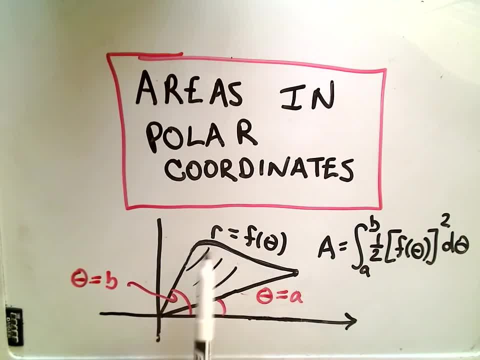 So again, remember things in polar coordinates. certainly the graphs are a little different, but suppose this is my graph: r equals f of theta. Again, where theta is our angle, r is the radius or the distance you go out from the origin. 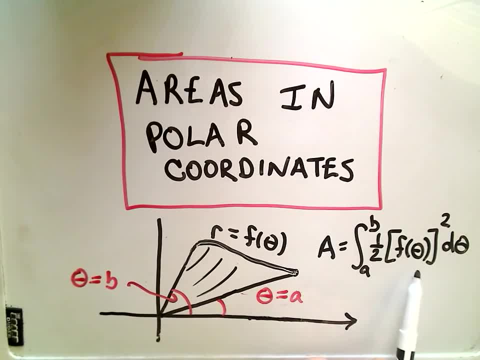 The thing that you integrate is pretty easy. You just take one half of the function squared. The parts to me that are usually a little more complicated are finding the limits of integration, And in this case again, the limits of integration correspond not to these rectangular intervals. 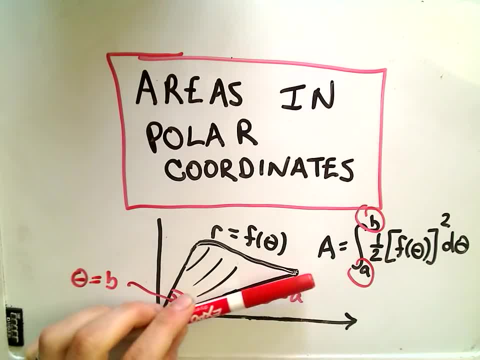 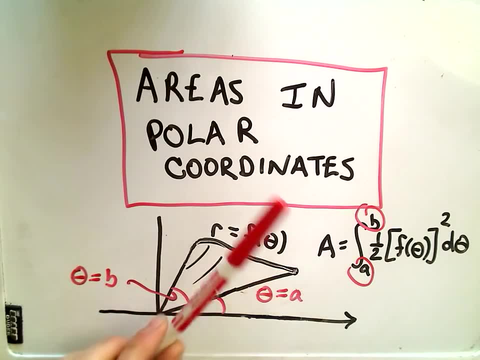 like when we do normal integration, but now our limits of integration are going to be angles. Okay, so suppose it starts at theta, It goes to the angle theta equals a and goes to the angle theta equals b. Those are going to be my limits of integration. 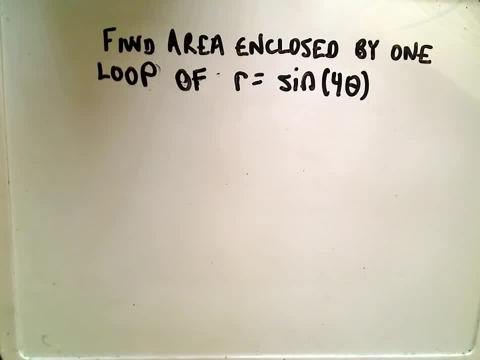 So let's do one simple example. In another video I'm going to do one where you've got to find areas enclosed by two different curves, So this will certainly be the more simple of the two. It says: find the area enclosed by one loop of r equals sine 4 theta. 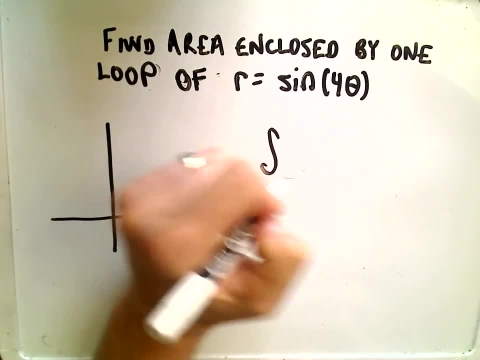 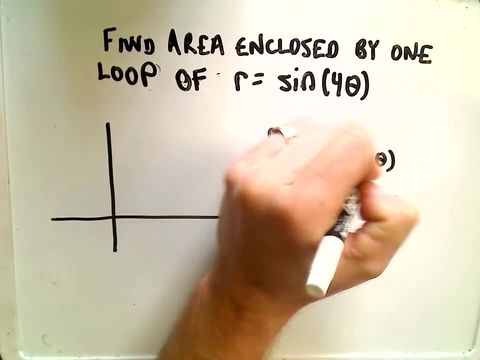 Okay, so I'm going to try to come up with a decent little graph. I already know that it's going to be one half and I have to integrate sine of 4 theta. This is the function I have to square. So there's the square d theta. 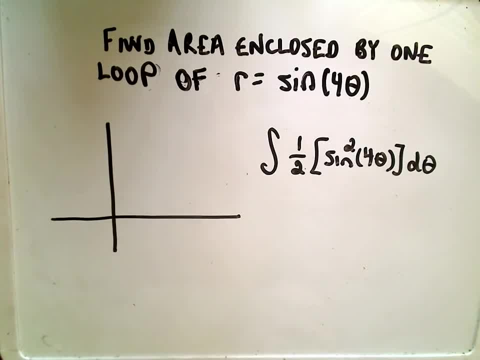 Now the only thing I really have to work for, at least in this simple example again, are the limits of integration. The way that I do this, you know kind of a quick way that helps me find the graph of this thing. 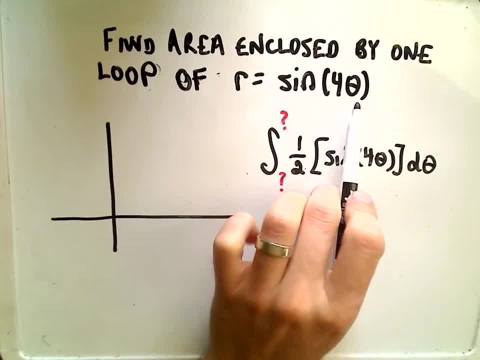 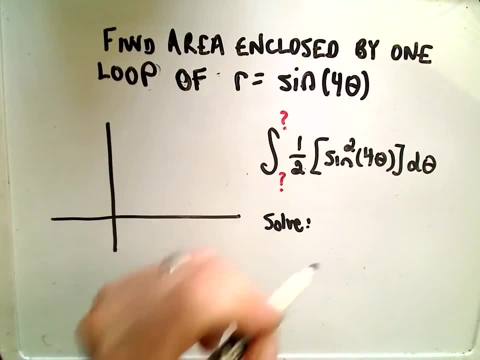 is what I'll do, is I like to figure out for what theta values does the radius equal 0?? So really, for me, to help me get a graph, I'm just plotting points. I like to solve this equation. Okay, so I want to know what values of theta I get a radius of 0 out. 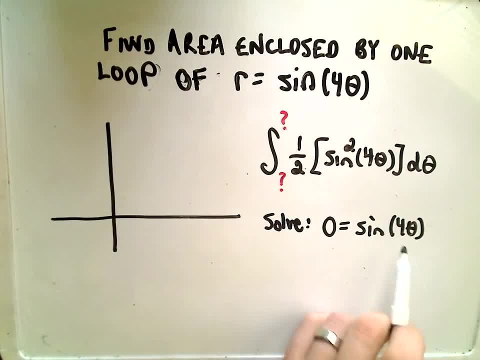 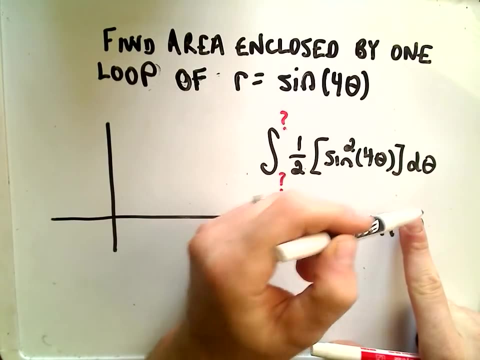 Well, if you think about it, sine of well, let's see, 0 would equal 0. Normally. so forget about the fact that there's 4 theta here. If the 4 theta wasn't here, the values we would like to have on the inside would be 0, pi, 2, pi, 3, pi, 4, pi, 5, pi, etc. 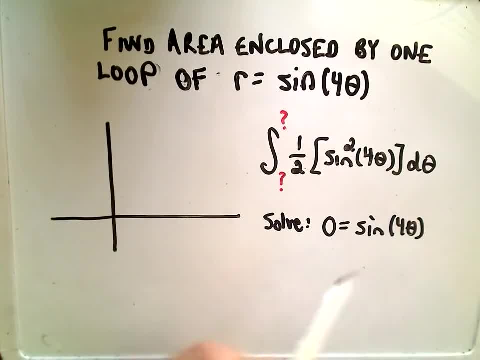 Sine of those angles equals 0. But obviously we're going to have to tweak that a little bit because of this 4 out front. Well, what it says again is: we would like the inside, the 4 theta. 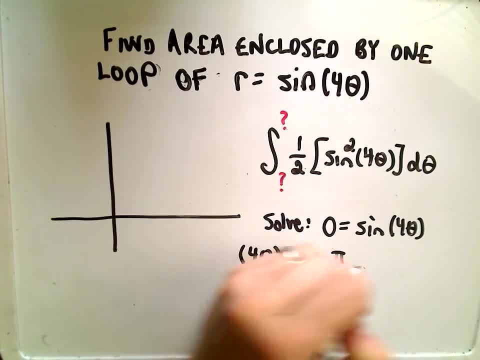 I would like that to either equal 0, or pi, or 2 pi or 3 pi, etc. When this happens, that's when I'm going to get sine of those corresponding angles, giving me a radius value of 0. 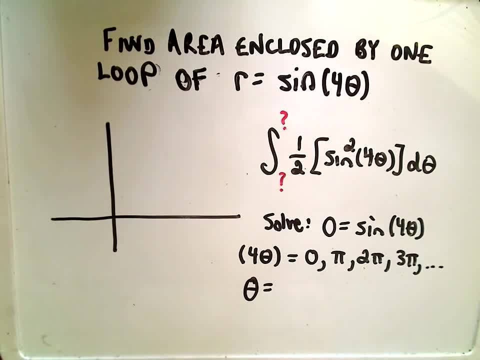 So this is going to happen then. well, you can imagine dividing both sides by 4.. This is going to happen at the angle. theta equals 0, pi over 4, 2 pi over 4, 3 pi over 4,, etc. 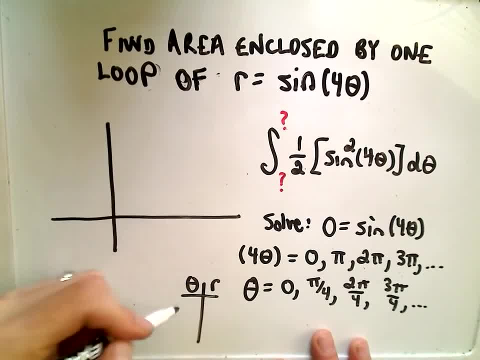 So really what I'm doing is I'm just plotting points. You know, here's theta, here's r. So now I know, at 0, pi over 4, 2 pi over 4, 3 pi over 4,, etc. 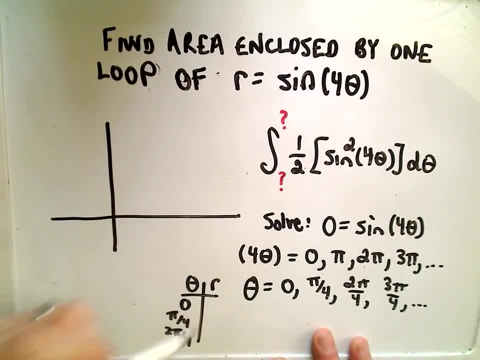 So really, what I'm doing is I'm just plotting points. You know, here's theta, here's r 2, pi over 4, etc. I know that for these angles, that the radius is always going to be 0. So why do I do that? 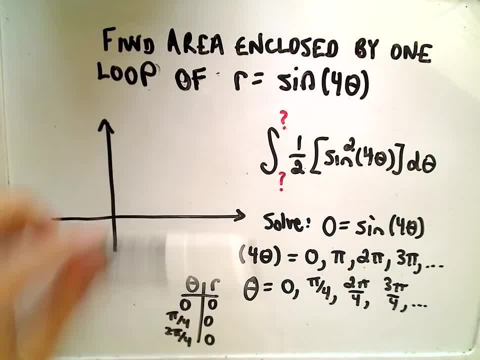 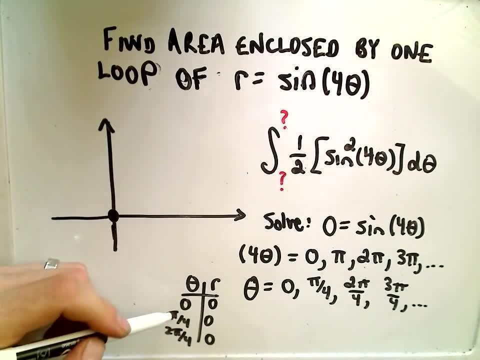 Well, it tells me then, when the angle of theta is 0, it says my radius value is 0. So I'm just sitting right here, Okay. so now let's think what happens. So I'm really now thinking about the interval. 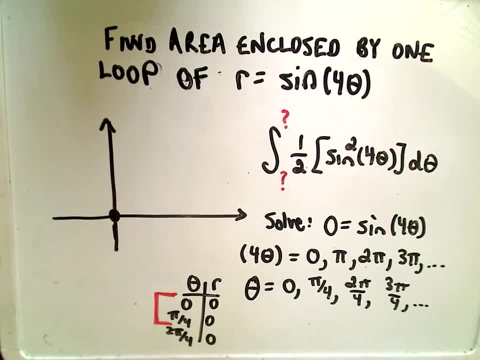 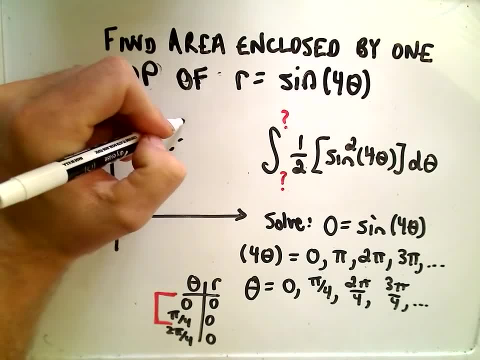 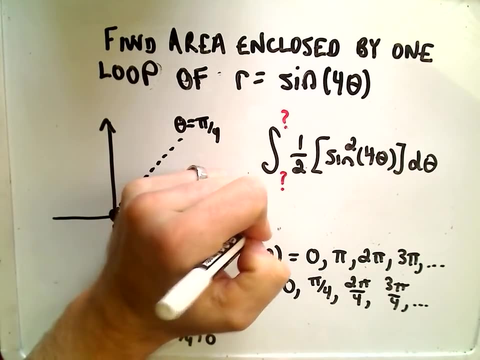 I'm thinking about theta values between 0 and pi over 4.. Okay, The angle pi over 4 is going to be this angle. So here's: theta equals pi over 4.. Again, the angle: theta equals 0.. That would just correspond to our x-axis. 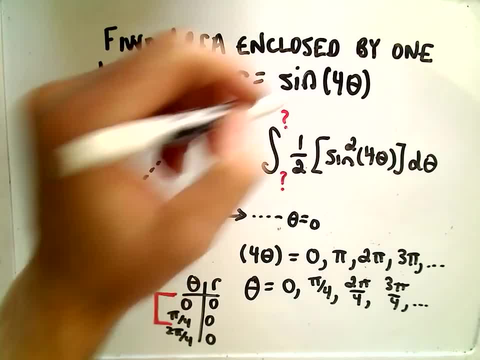 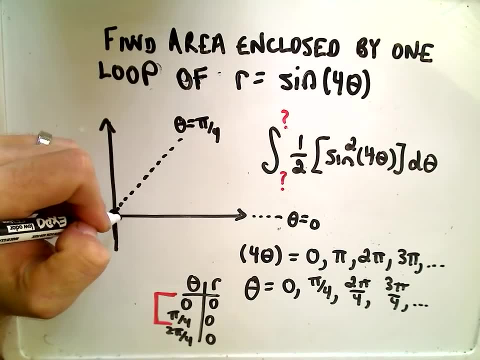 Notice this: theta increases Our value. well, 4 theta will increase. Sine for a little bit, will start getting bigger, bigger and bigger. I think you can justify that at pi over 8, you're going to be at its maximum distance away. 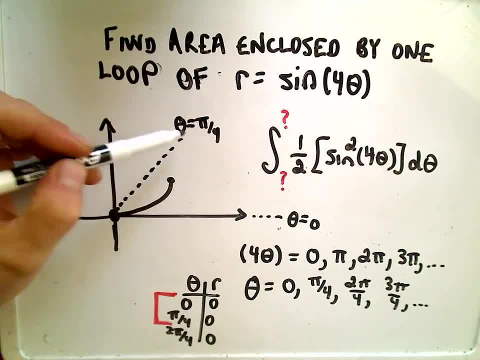 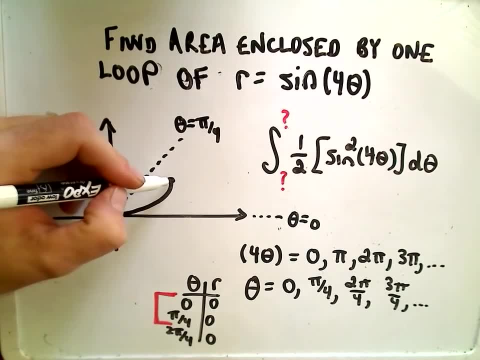 So, once we get out to an angle of pi over 8, which is halfway between, well, pi over 4 and the angle 0, it'll be at its maximum distance And then, as theta increases, from pi over 8 to pi over 4,. 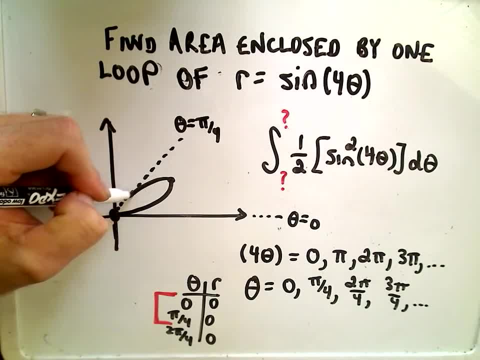 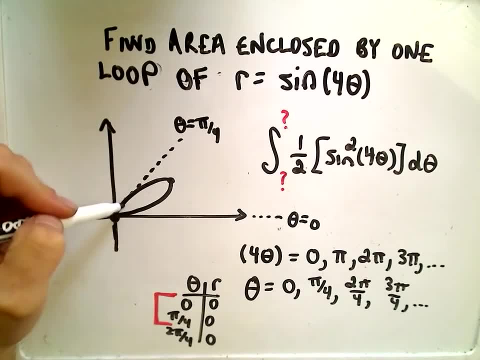 sine is going to start decreasing and it gets pulled back into this value of 0.. Okay, So basically I'm finding my limits of integration by doing. this is what I do. So again, this is kind of a quick little synopsis. 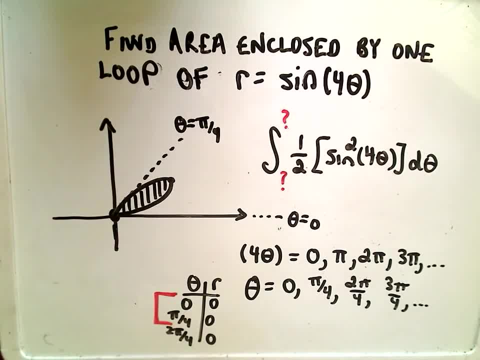 of graphing, you know graphing polar curves. So again I think that part can be pretty tricky. So to me as a student, that's the part that I certainly spent more time on was just the graphing, because again, I think once I got that 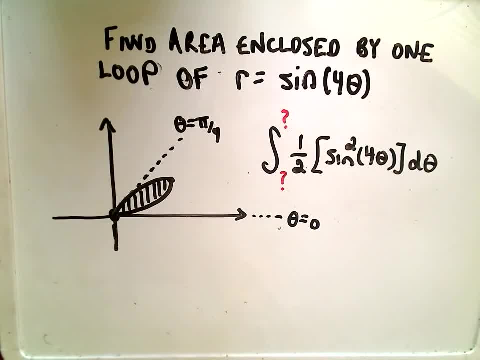 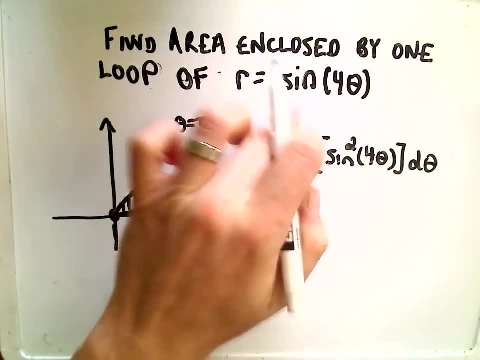 the limits of integration come from that. Okay, So, all right, so I think we've got it now. Our lower limit of integration is going to correspond to theta equals 0.. Our upper limit of integration is going to correspond to theta equals pi over 4.. 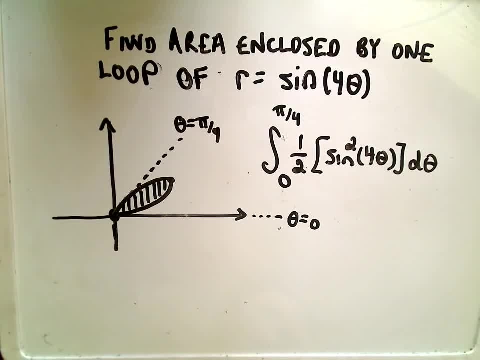 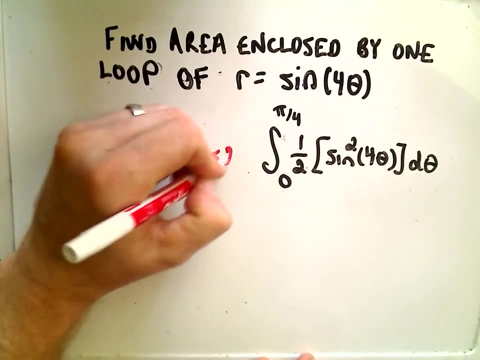 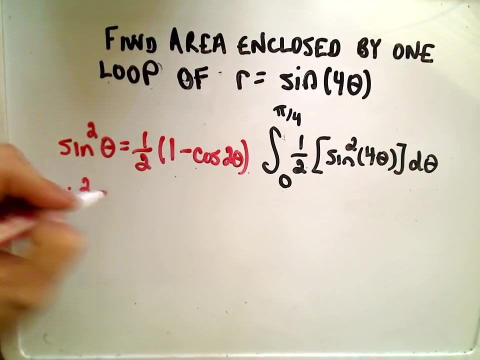 And now all I have to do is integrate away. So we're going to have to use one little identity here. Remember, there's an identity. It says: sine squared of theta equals 1 half 1 minus cosine of 2 theta. So to integrate sine squared 4 theta, equivalently, I can write sine squared of, well, 4 times theta. 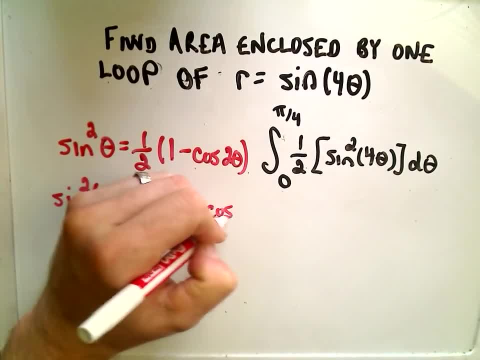 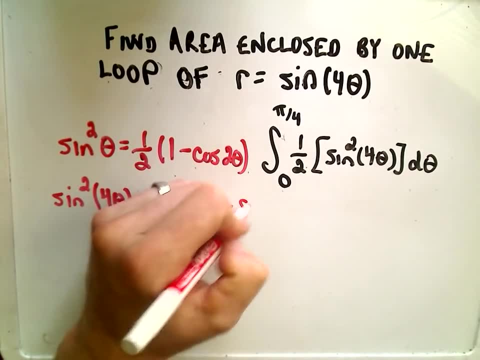 That's going to be 1 half of 1 minus cosine of 2 theta. Notice it says: whatever theta is on the left, you double it on the right. We have 4 theta here, so I'm going to get 8 theta here. 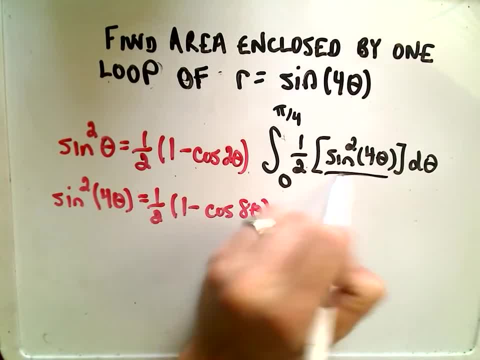 Okay, So this is the identity I'm going to use on the sine squared of 4 theta part. to kind of break it up: Okay, So when I integrate I'm going to pull my original 1 half out front. So there's the 1 half that just comes from the formula. 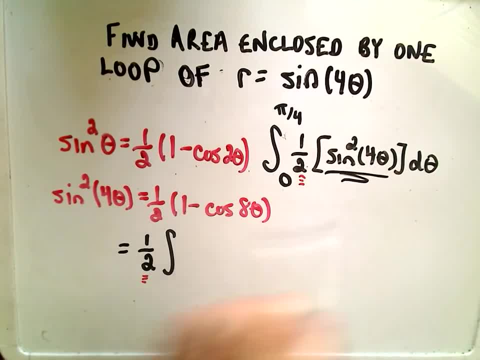 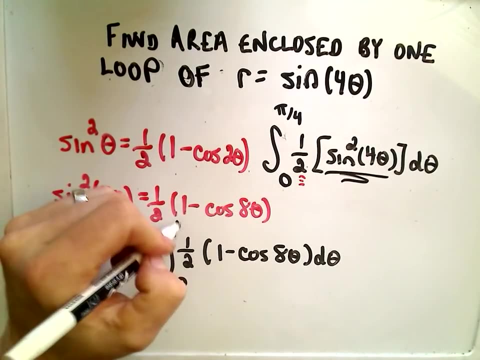 And now, when I use my trig identity on the sine squared 4 theta, I'm going to get all this stuff. I'm going to get 1, half 1 minus cosine of 8, theta, d, theta. And again we have to integrate this simply from 0 to the value pi over 4.. 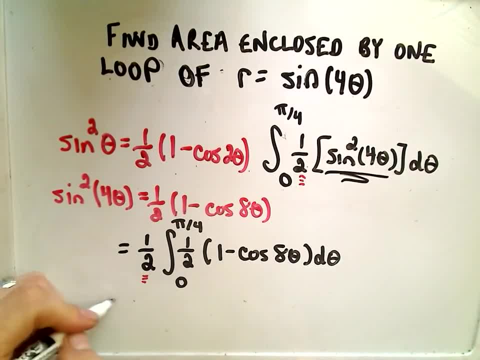 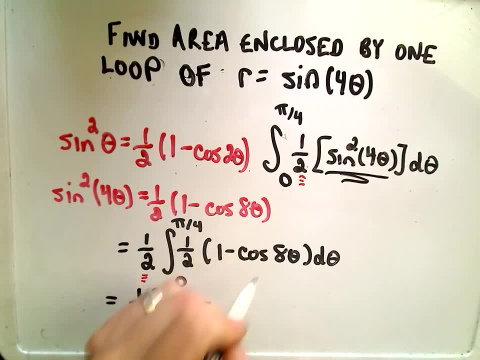 So okay. so now it's just tedious integration. I'm going to multiply the two- 1 halves and get a fourth. If I integrate 1, I'm going to get theta, The antiderivative of cosine 8. theta is going to be sine of 8, theta over 8.. 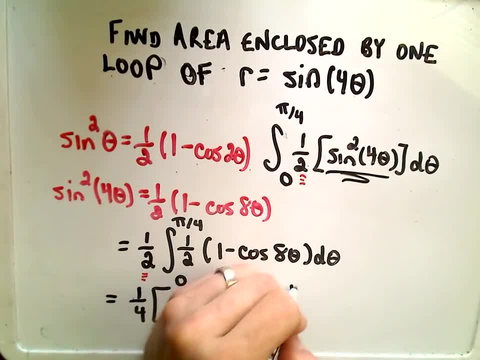 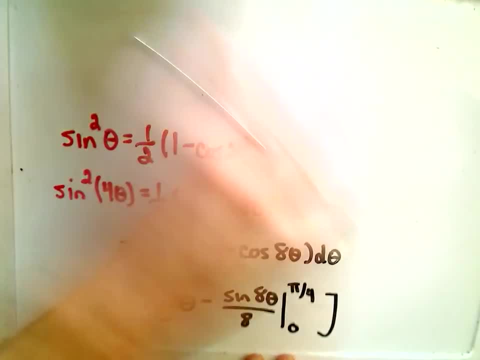 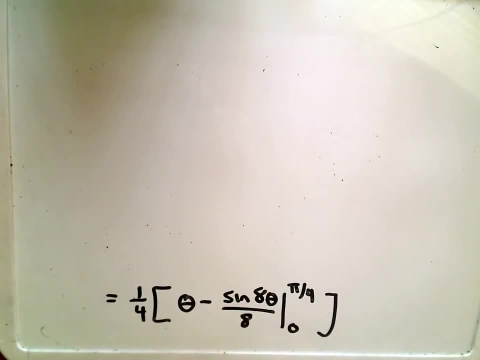 You can justify that Using a u-substitution. We have to evaluate this from 0 to pi over 4.. So let's go ahead and do that real quick. Again, we're finding areas here, So you know you better get something positive out or something went wrong. 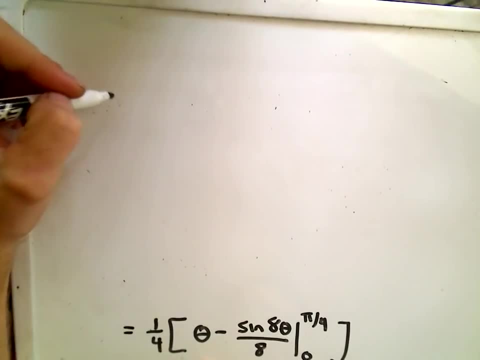 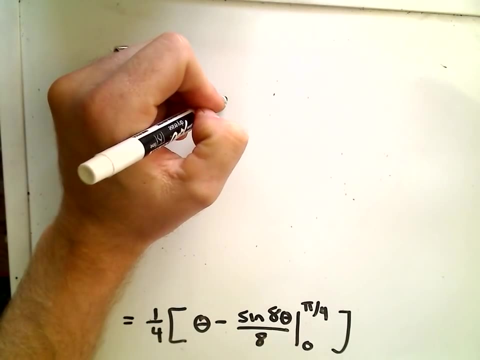 Let's see here. Okay, So let's plug everything in. So we're going to have 1. fourth, I'll plug in pi over 4.. I'll have to subtract away Sine of 8 times pi over 4.. 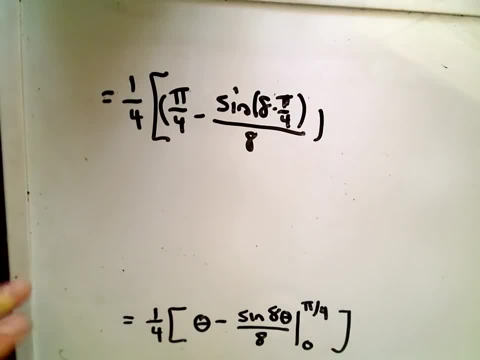 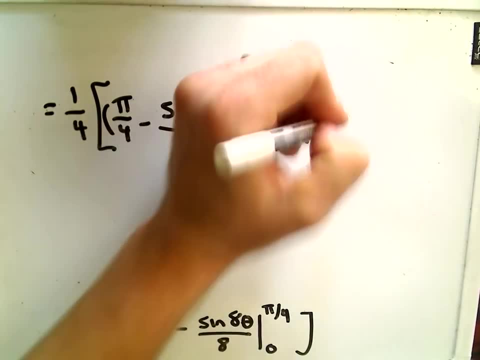 Again, that's all being divided by 8.. There's my upper limit of integration, And then we'll have to subtract away the lower limit. So if I plug in 0, I'm just going to get 0.. Notice: on the inside, 8 times 0 will be 0. 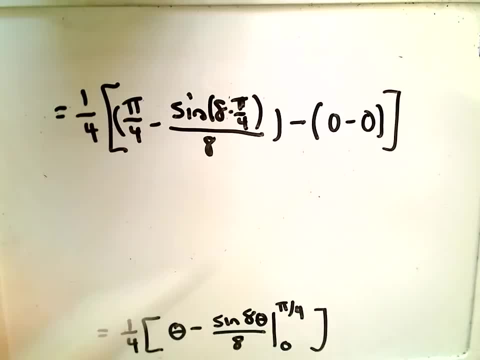 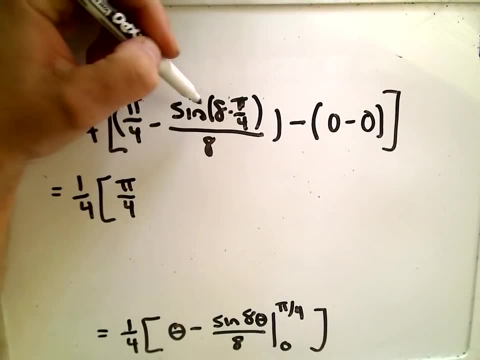 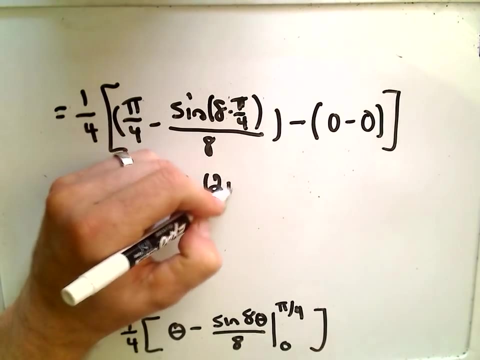 We know that sine of 0 is 0. So the lower limit just turns into 0s. So we're almost there. Pi over 4 is just chilling. Notice 8 pi over 4. That's 2 pi. So really we get sine of 2 pi divided by 8.. 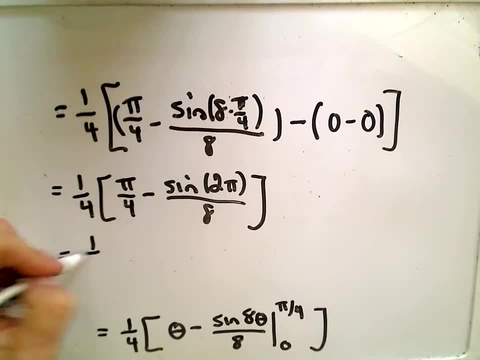 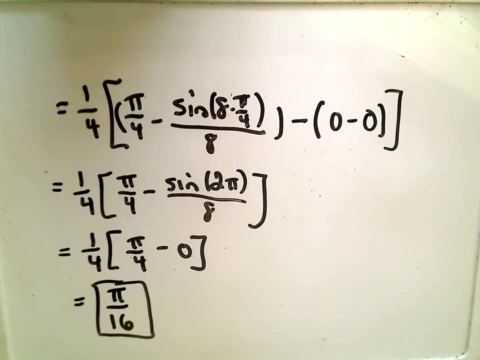 But likewise sine of 2 pi is just equal to 0. So if we multiply it looks to me like we get the value pi over 16.. All right, So I hope this video made some sense. Again I've got videos on grammar.